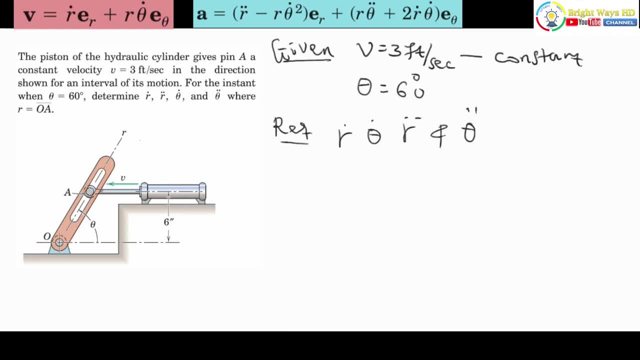 of this, and then the other parameter is here. we know that one feet is 12 inch, so here is a 6 inch. so if we convert it into feet it will become 0.5 feet, because we have to change every parameters into the same unit. once we have this, let's just try to find out the radius r of the point from. 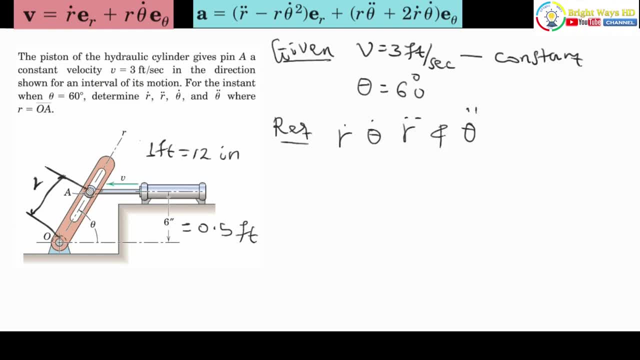 o up to a. that's r here. so this can be evaluated from the trend angle for any triangle. if this is theta and then if this is 90 degree- now we know that this is 0.5 feet- and then this is r. the theta is given here is the 60 degree. so r times sine, 60 degree is. 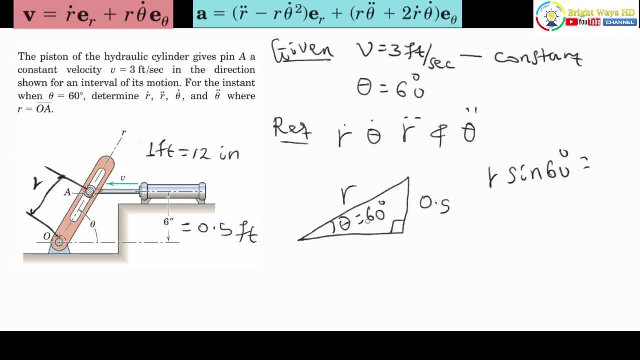 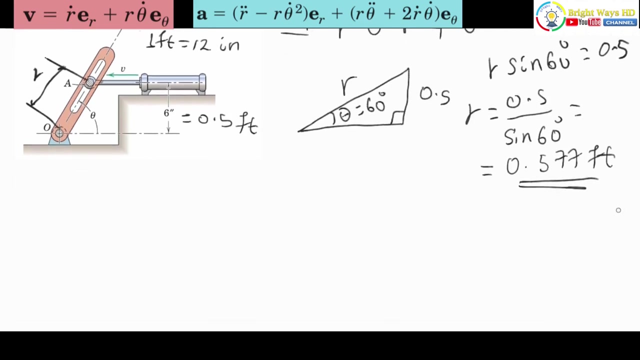 equals to the opposite sides of the angle and in will become 0.5. that means r is equals to 0.5 over sine 60 degree, and then it will become 0.577 feet. this is the r parameter for this position and then the other one. once we have do this, we know. that the velocity is 0.577 feet, and then the other one. once we have do this, we know that the velocity is 0.577 feet. this is the r parameter for this position- and then the other one. once we have do this, we know that the velocity is. 0.577 feet. this is the r parameter for this position, and then the other one. once we have do this, we know that the velocity is 0.577 feet. this is the r parameter for this position, and then the other one. once we have do this, we know that the velocity is. 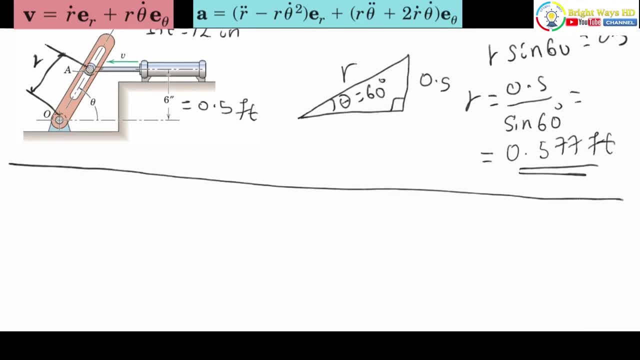 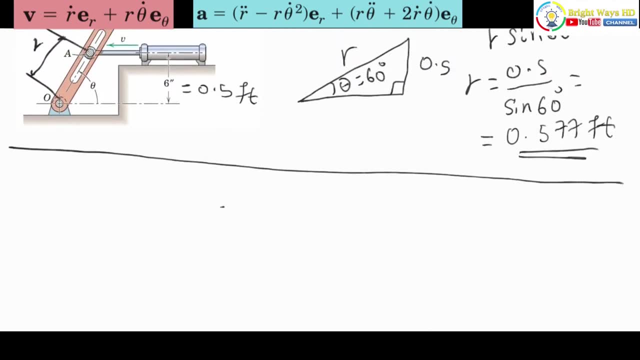 0.577 feet. this is the r parameter for this position and then the other one. once we have do this, we know that the velocity is in the left direction. now for evaluating the r and theta components of the given velocity, we can decompose it into this intended directions. this one is er, and then this is the perpendicular. 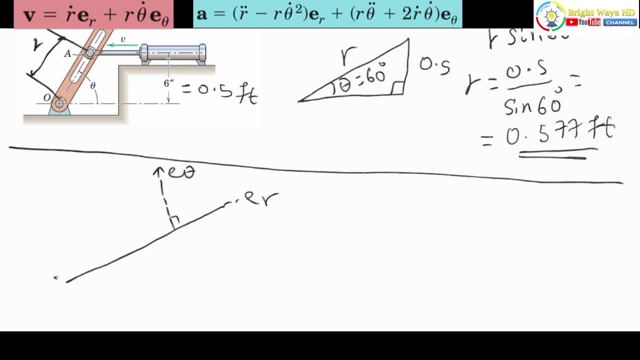 one. and then this is e theta direction. and from the horizontal we know that this is 60 degree. that means if it is 60 degree it will become also 60 degree, and then this one will be 90 minus 60, and then this 30 degree, and we know that the velocity is in this direction. the theta components: 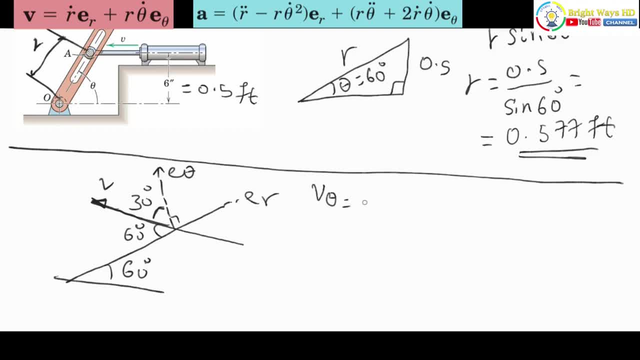 of the velocity v theta is equal to v times cos 30 degree. this implies that velocity is three feet per second times cos 30 degree. you, and then finally v theta will become 2.6 feet per second, then the other one, the other components of the velocity will be evaluated with this one, so v in the r direction will be equal to. 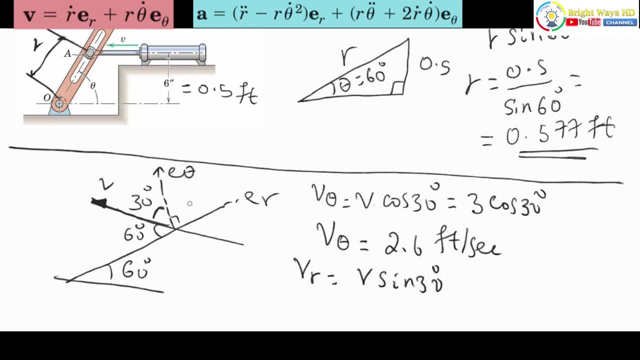 v times sine 30 degree. but in which direction? if you look at the direction, this one is a negative er direction. So this velocity component will be decomposed into the negative direction because the positive one is greater than 180 degree. So it will be negative. 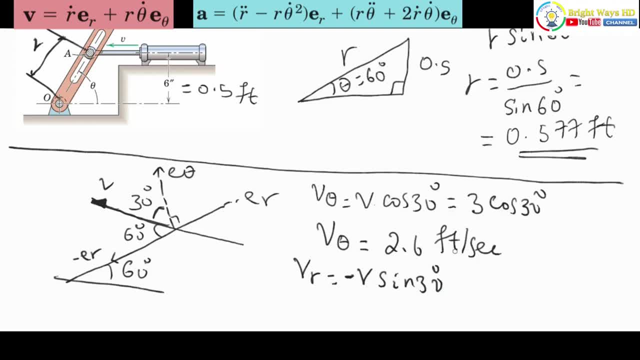 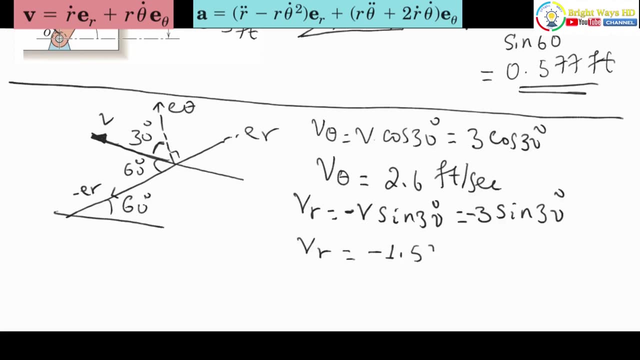 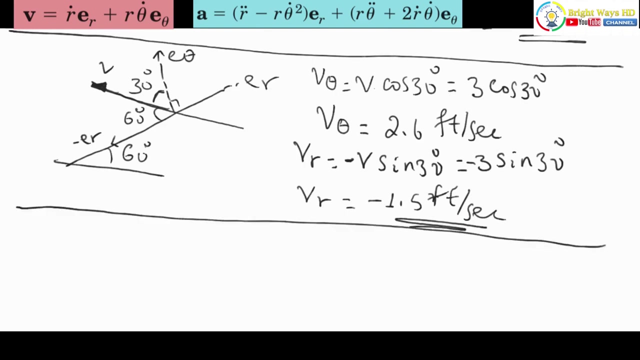 So negative times V sine 30 degree will be velocity in the R direction And then it will become 3 times sine 30 degree negative And then V? R will become minus 1.5 feet per second. Once we evaluate them, we can easily evaluate theta dot and then R dot. 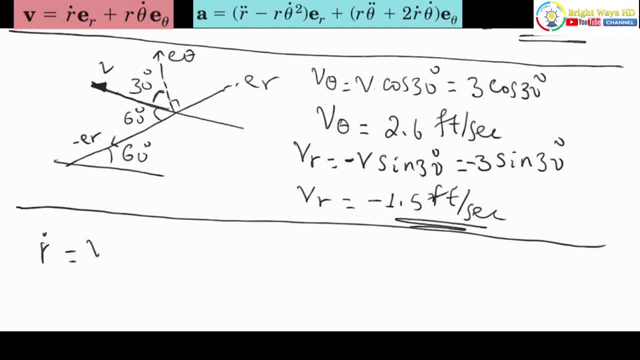 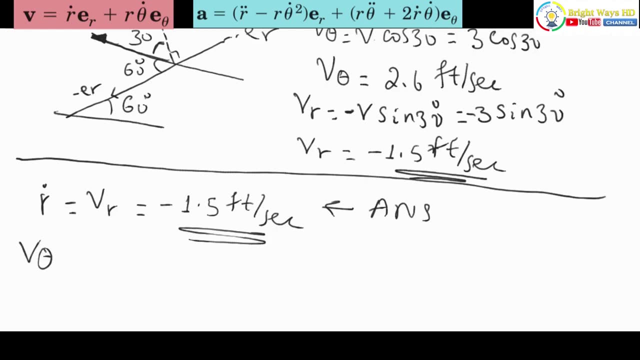 Normally R dot is equal to V in the R direction, and it is evaluated here, so it will become 1.5 feet per second. This is Our answer. And then for theta dot, we know that velocity in the theta direction is equal to R times theta dot. 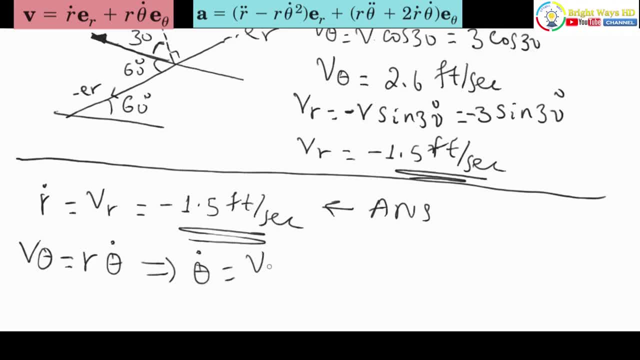 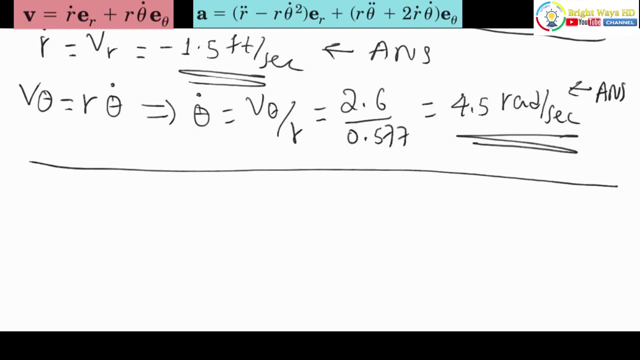 Which means theta dot is equal to V. theta over R, And then it will become 2.6 over R is 0.577. And then, finally, theta dot become 4.5.. Rad per second. This is the answer Evaluating R double dot and theta double dot. we have to evaluate the acceleration in the R direction and in the theta direction. 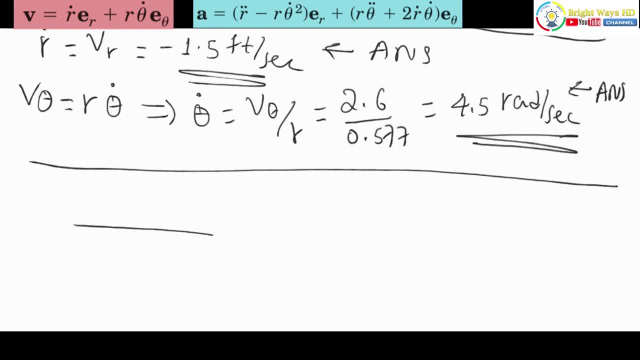 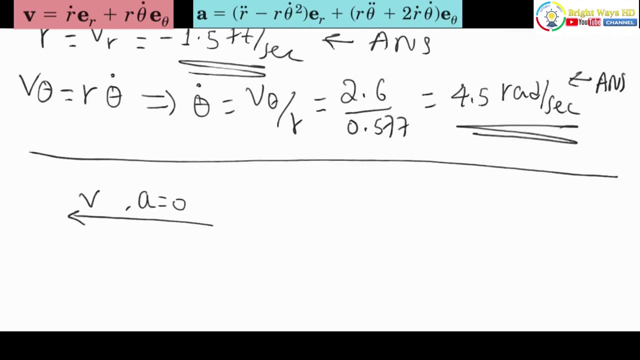 Let's do that one now. If you look over here, the velocity is constant in this direction. That means if the velocity is constant, there is no any acceleration in this direction. So the acceleration will be 0. So the only accelerations will be on the vertical axis. 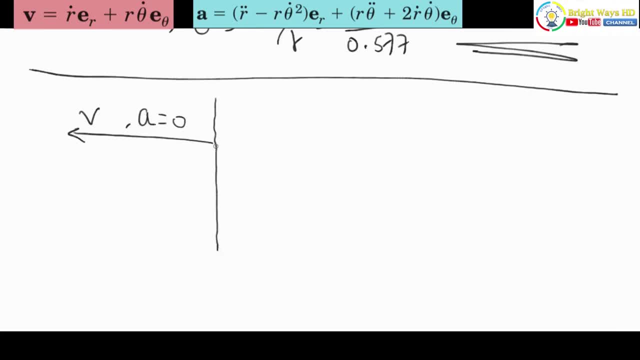 So if that is the vertical axis component, Now if you just Redraw the previous diagram, We know that This one will be the normal direction E in, And then for the particle in the perpendicular to this one, We'll have a tangential direction Et. 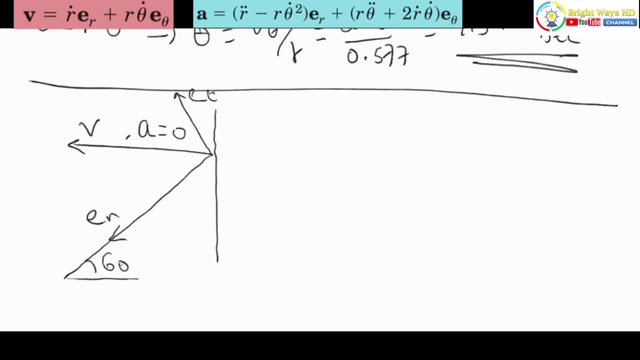 we know this is 60 degree. but here, if you remember from the normal tangential coordinate system, the acceleration in the normal direction is always toward the centers of the curve and then it will become an here, so an is in the directions toward this, the center, that means to be in this direction, so an is. 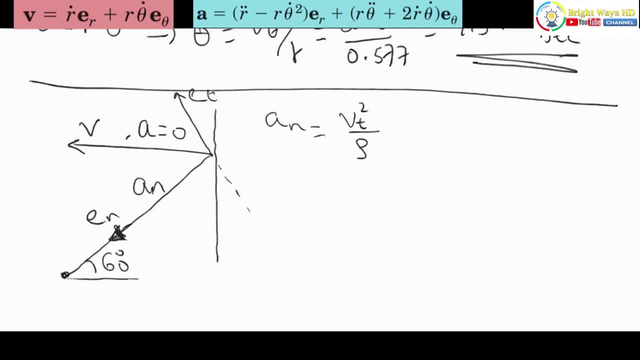 equals to tangential velocity. square over a row and then the tangential velocity is equals to V theta and it is 2.6. so 2.6 the whole, square over 0.577 and then it will become 11.7 feet per second squared. we know that there is a 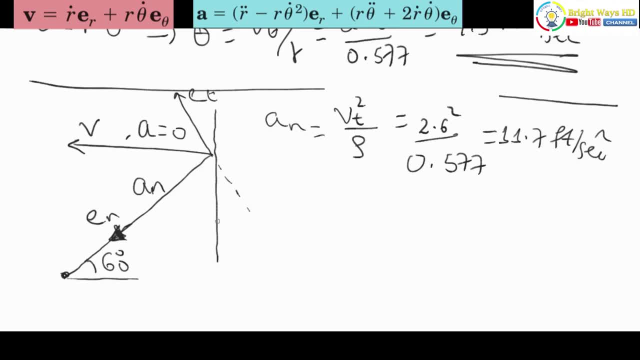 component of the normal acceleration here. and then, where will be just the magnitudes of the acceleration? is it in the positive direction or in the negative direction? so the the vertical axis, obviously, since this component, the normal acceleration component, over this one, that means over the 60 degree inclination, will have some 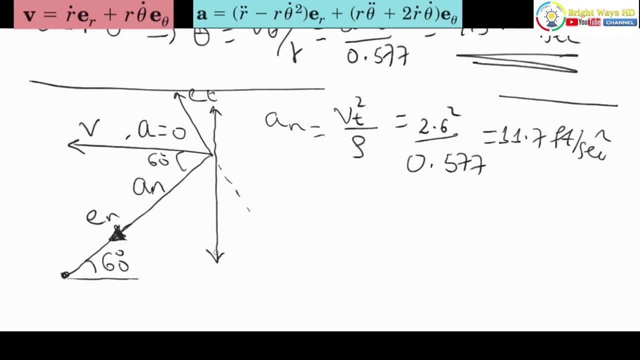 positive values here. that means it will have in this direction. so acceleration will be equals to an in the n direction plus a tangential in the 80 direction. since the normal acceleration will be will have a positive value here if the directions of the tangential acceleration is in toward this, in this positive 80 direction. that means both. 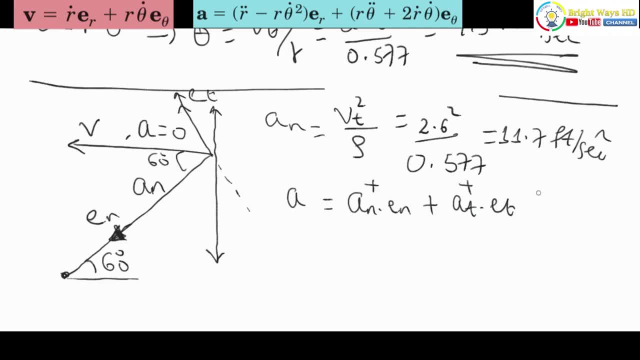 values will be positive and then if you sum up them, they will be greater than zero. but if you know from the previous concept, the velocity is constant and there is no acceleration. this direction, that means the only option that can be the tangential acceleration, will be in the negative tangential direction. that 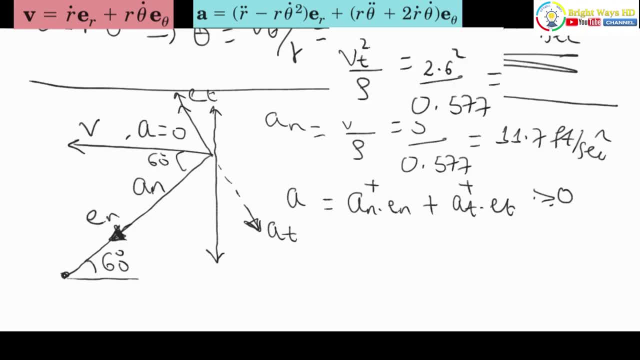 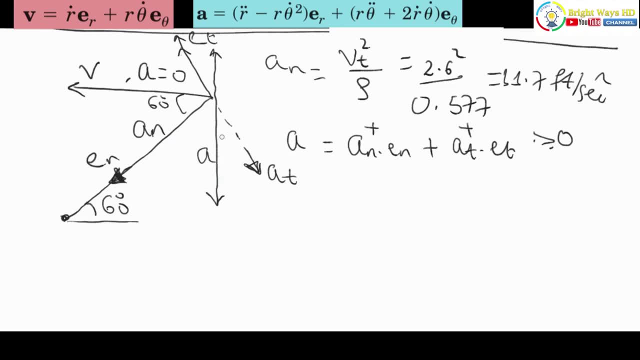 means it will be in this way. so once we get the normal acceleration, this one will be the magnitudes of the acceleration in the negative vertical direction and then, if we decamper, this one will be 90 degree and in this part, toward these directions, will be tangential acceleration. and then this: 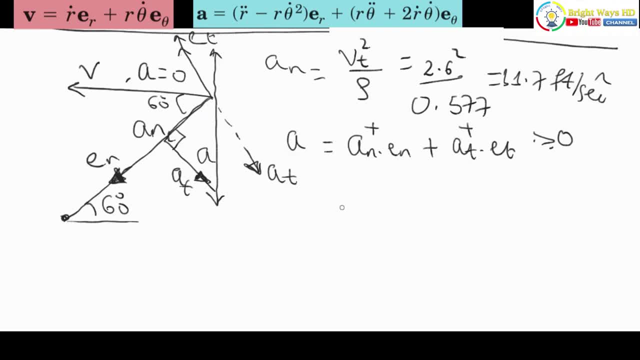 one will be a normal acceleration. that means, if we take out this diagram, we will have an acceleration in this way, a normal acceleration in this direction, and then a tangential acceleration this direction. this is perpendicular to each other. and then we know that this is 90 degree, so it will become 30 degree. 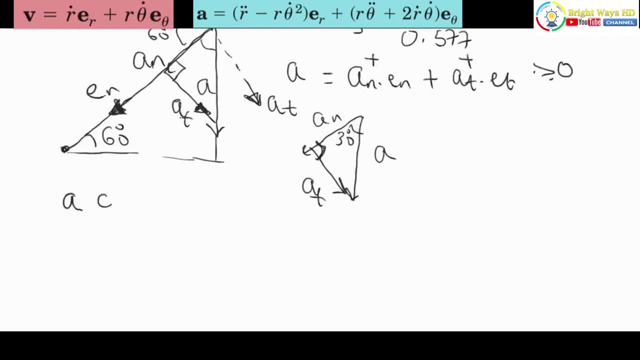 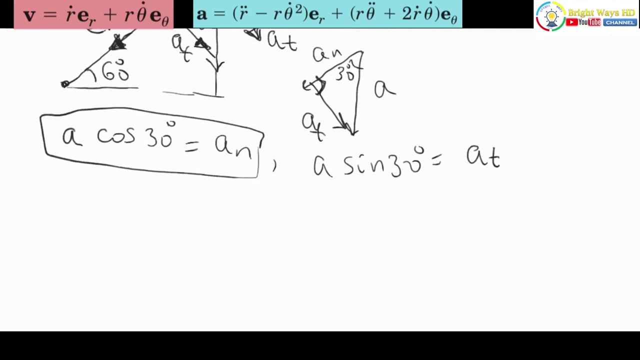 acceleration times cos 30 degree is equals to normal acceleration and acceleration time sine 30 degree will be equals to tangential acceleration. from the first equation here we can evaluate the acceleration. acceleration will become normal acceleration divided with cos 30 degree and then it will become the normal acceleration is evaluated here is 11.7. so 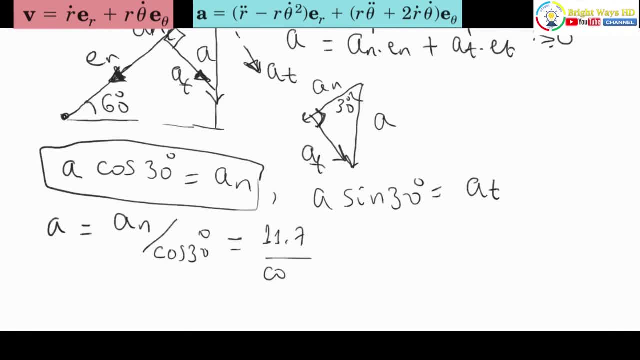 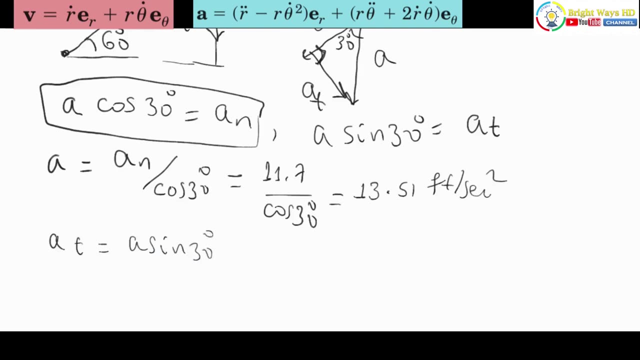 11.7 divided with cos 30 degree, and then it will give us 13.51 feet per second square, and the tangential acceleration is a times sine 30 degree, which is equals to 13.51 times sine 30 degree, and then it will become 6.755 feet per second. but what about the directions of? 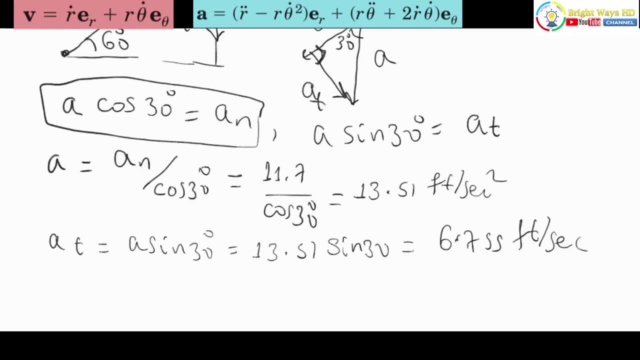 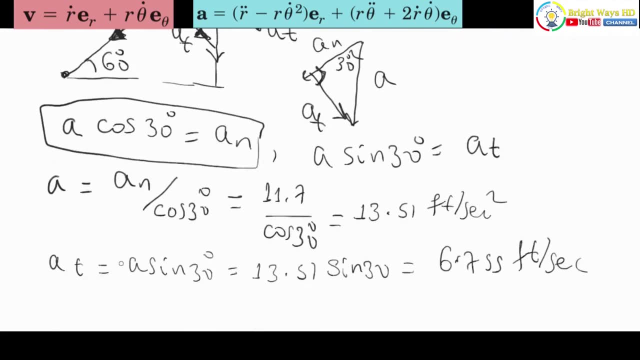 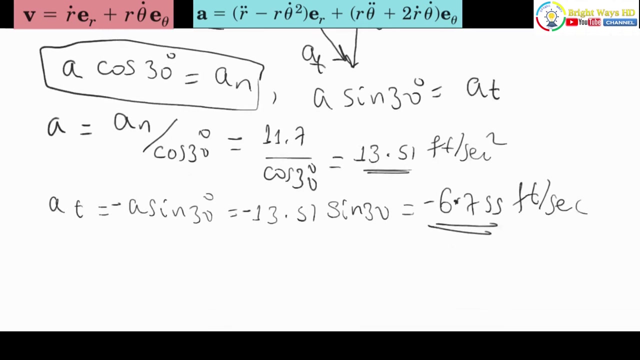 the tangential acceleration. is it positive or negative? since it is in the negative ET direction, the tangential acceleration is negative. that means it will be the negative sine tangential acceleration will be negative, 6.755, and then the total acceleration is 13.51 feet per second squared. now, once we have 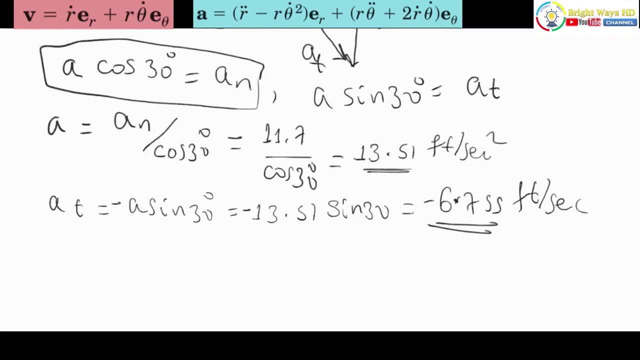 this we can evaluate r double dot and theta double dot from the polar coordinate system. we know that acceleration in the r direction is equals to r double dot plus r times theta dot squared. this implies that r double dot is equals to AR minus r theta dot squared. 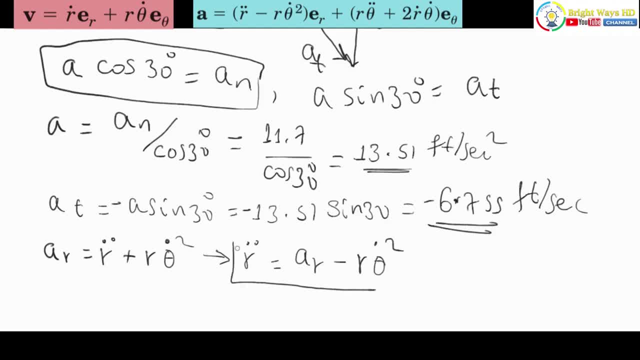 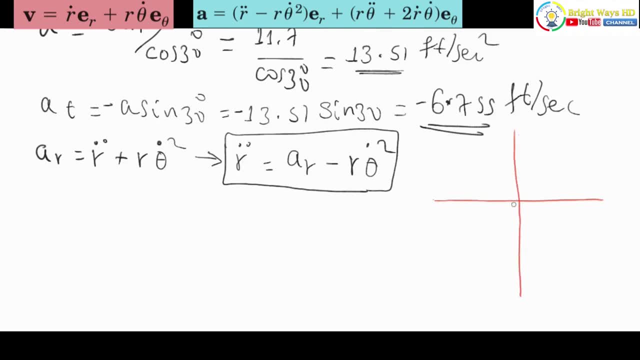 we substitute the numerical values, we can get the r double dot. if we just decompose it, the directions, into this way, we know that this is EN direction and then at the core linear line we will have ER direction and this is perpendicular to this axis. this is: 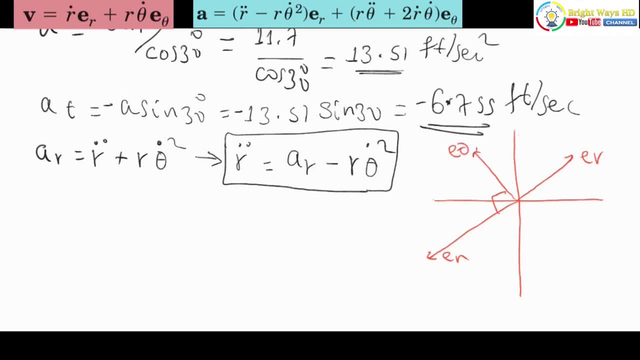 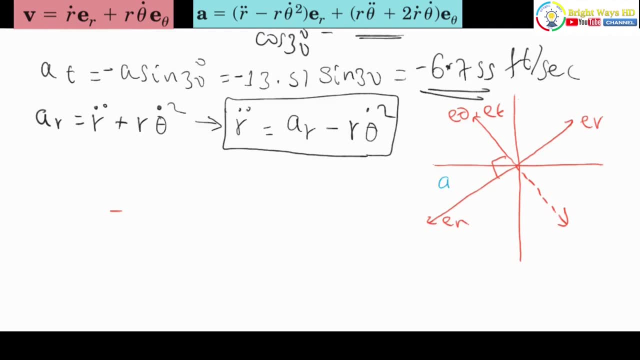 E theta direction and then at the same time it is a tangential direction. That means we know that this is AN and this is A tangential For polar coordinate system, this is A theta and then in this direction we will have AR. If you look over the graph, AN and AR are the same but in different direction. that means 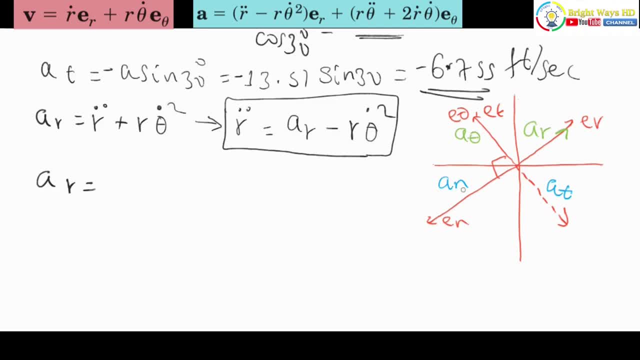 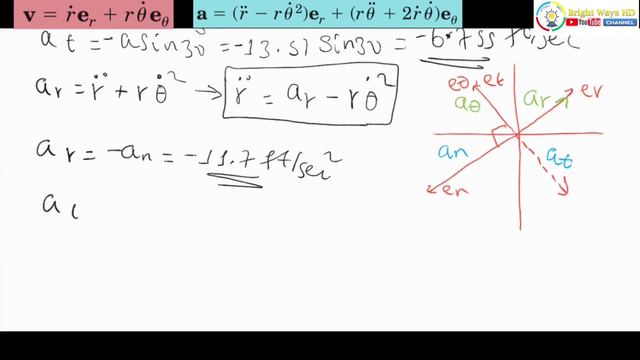 AR is negative, AN it will become negative, 11.7 feet per second square. and the other thing. if you look for A theta direction- since we are considering A theta as a positive in this way, but it is on the negative direction- that means it is in the negative E theta direction. 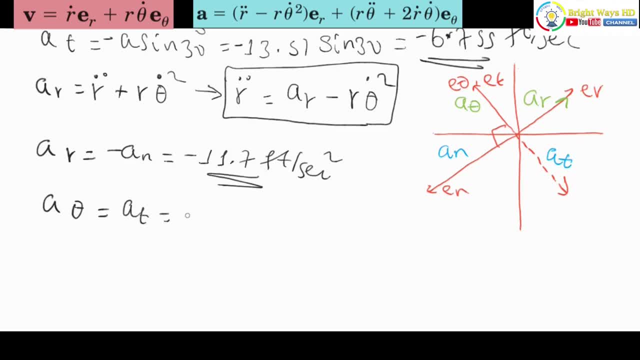 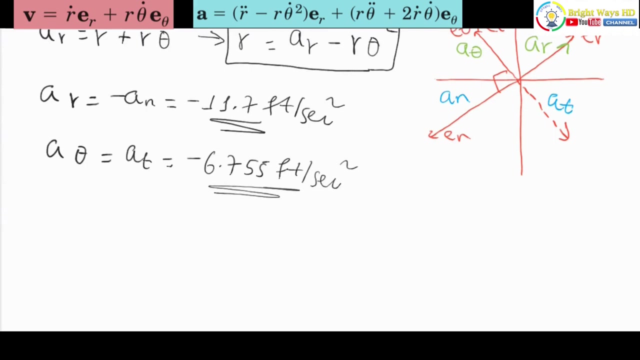 so it will become. It equals to 80, and then it is negative: 6.755 feet per second square. Now, both the accelerations are negative with respect to the polar coordinate system. Once we evaluate them, we can simply calculate R double dot and theta double dot. 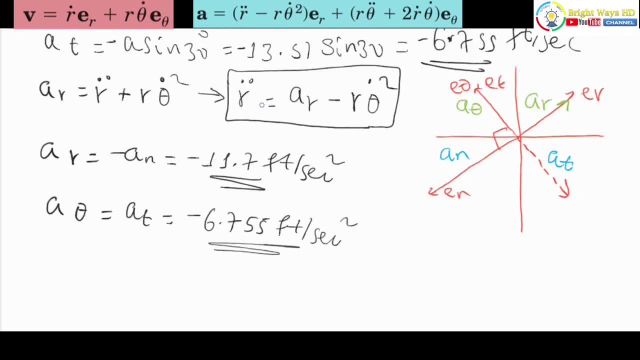 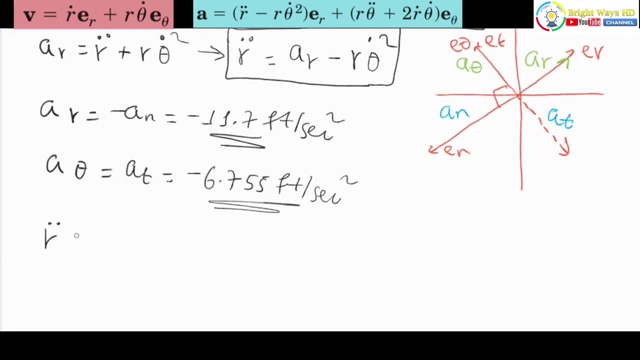 From a polar coordinate system. we know that R double dot is equal to AR minus R theta dot squared. That means R double dot will become, once we put the numerical value, it will become 11.7 minus 0.577 times 4.5 squared. and then it will become: oh sorry, we just make some mistake. 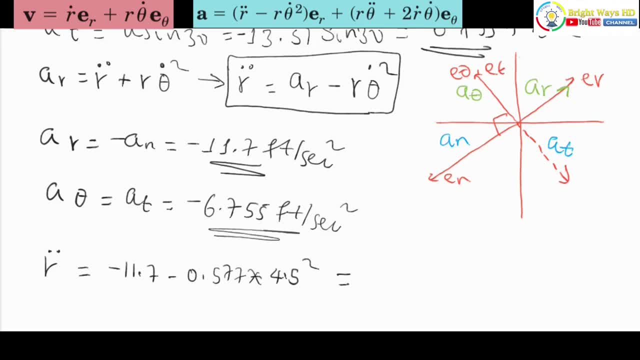 here. this is not a plus sign. this is a minus sign. That means AR will be R double dot minus R theta dot squared, which means R double dot will be AR plus R theta dot squared. that means it will be a plus sign. Once we substitute the numerical values, we can get negative 1.83 feet per second square. 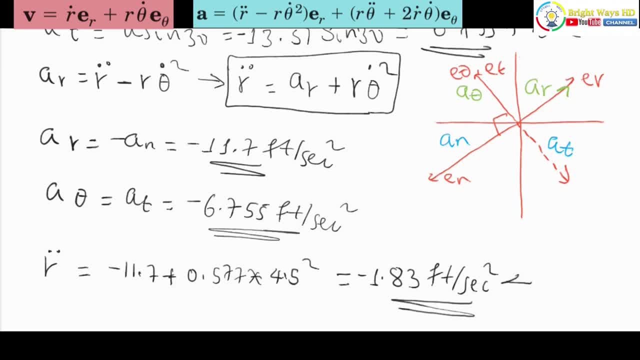 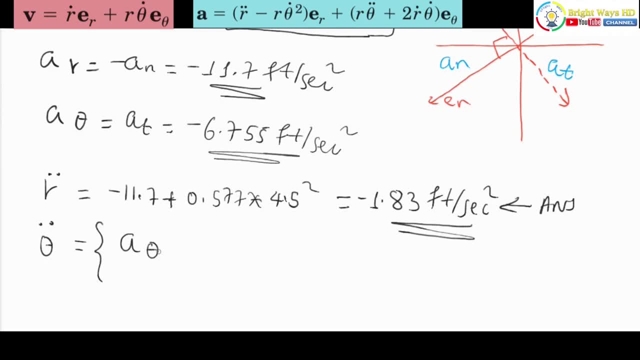 So this is our answer, Thank you. And then for theta double dot. for this part, let's see this: acceleration in the theta direction is equal to R theta double dot plus 2 R dot, theta dot, which means theta double dot will be equal to A theta minus 2 times R dot, theta dot squared. 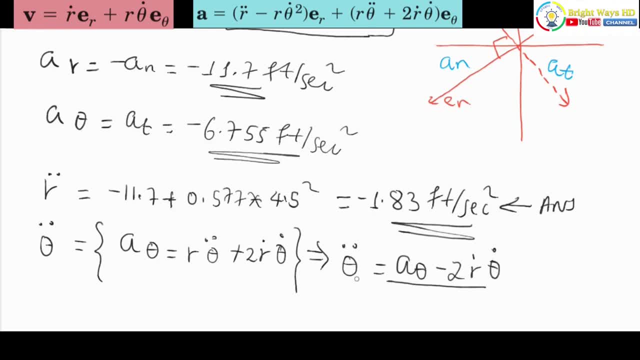 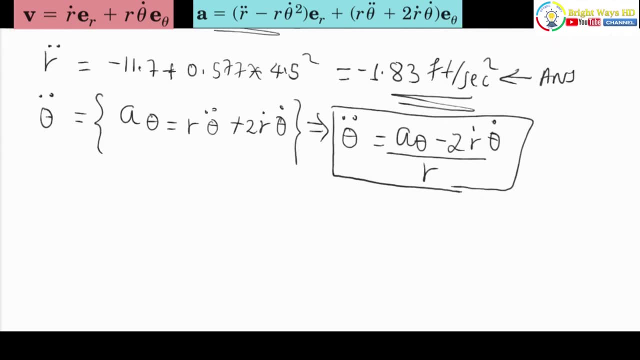 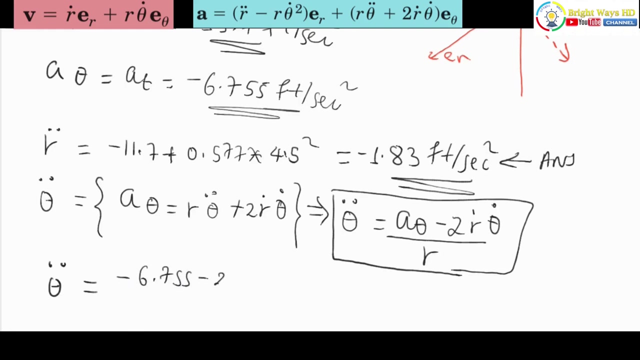 That means R dot. theta dot over the coefficients of theta dot is R, So theta double dot can be evaluated with this equation. Now the only thing is just substituting the numerical values. That means theta double dot will become A. theta is negative: 6.755 minus 2 times R dot. and then R dot is minus 2.755.. That means R double dot is equal to A theta minus 2 times R dot, theta dot squared. That means R double dot is equal to A theta minus 2 times R dot, theta dot squared.